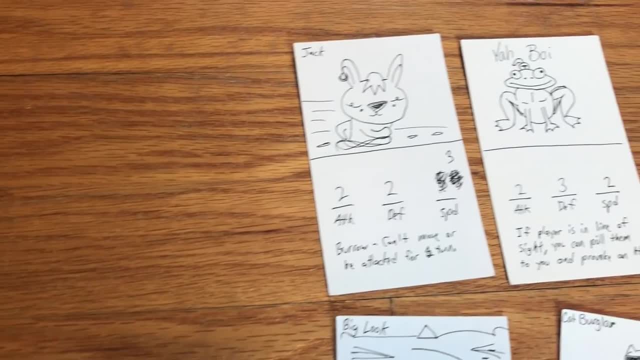 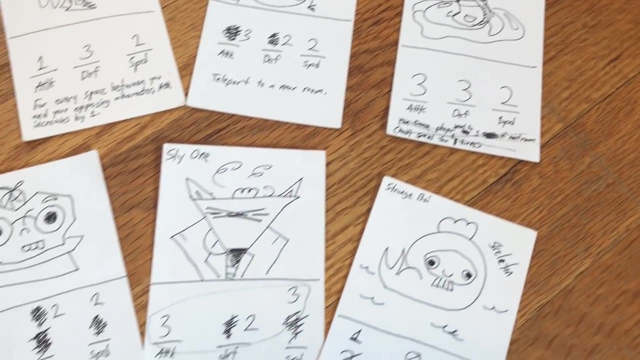 little bit intimidating because I didn't really know what went into making a board game. So I created a little mock-up using some index cards and actually played it with one of my family members. I remember them being incredibly confused and frustrated because I didn't know the rules and I literally was. 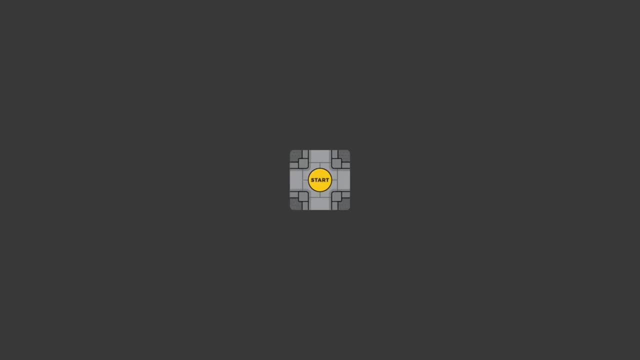 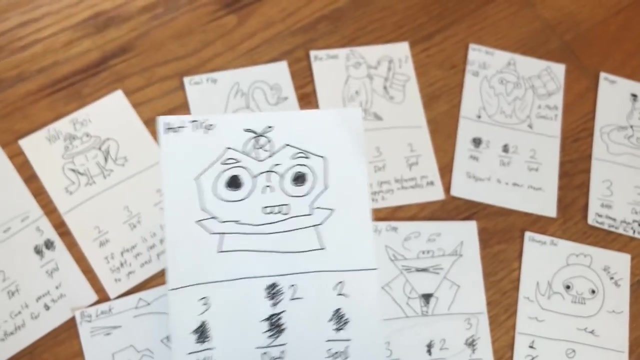 making up as I went on. One of the core mechanics I had for this game was that you'd actually build out the dungeon as you would explore it, And since I didn't figure out how movement worked or how many spaces you can go, let's just say 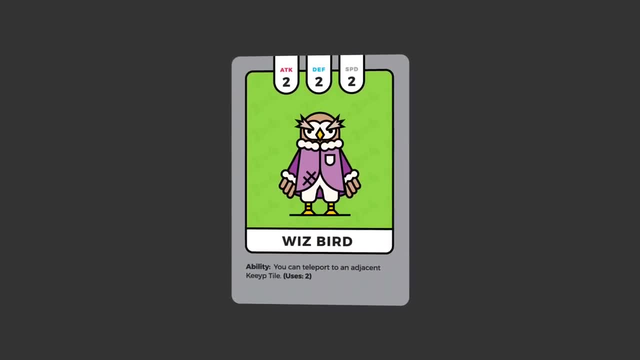 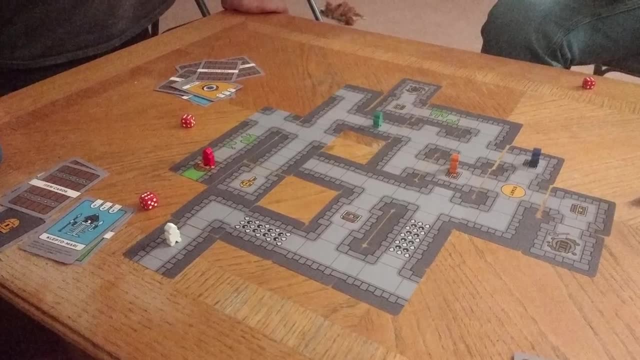 that the first round of the game was completely busted. So after learning what I didn't want in my game, I went back to the drawing board and tried to think of a new core mechanic. But that weekend I was meeting up with some friends and one of 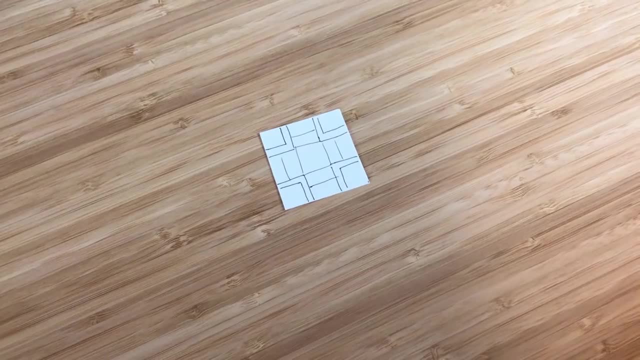 them kind of mentioned the idea of what if I brought the game and we'll test it. I thought that was a great idea. so I scrambled to rework the game to make it a little bit more playable for the group. When Friday rolled around, me and three 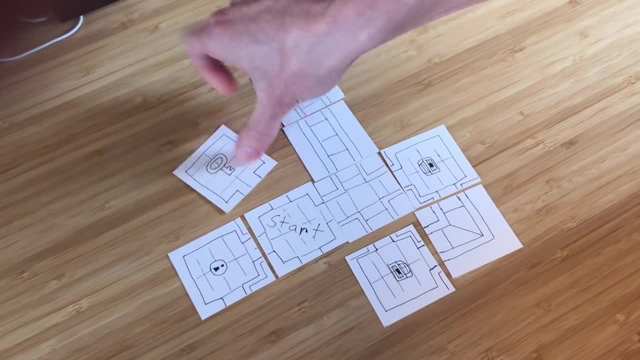 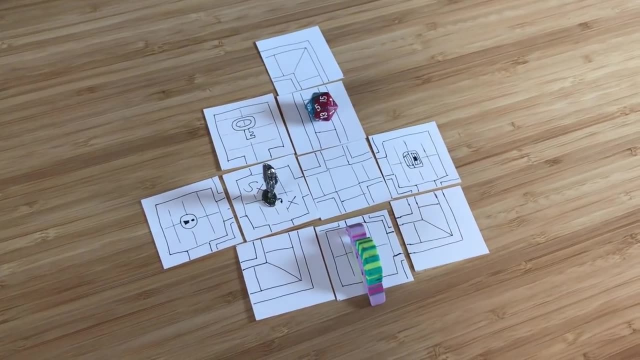 other. my friends met at a local coffee shop and played the game for a couple hours. I was actually surprised to see how this crude mock-up of the game actually became something fun and playable in front of my eyes By the end of the night. we actually figured out a lot of interesting mechanics that we 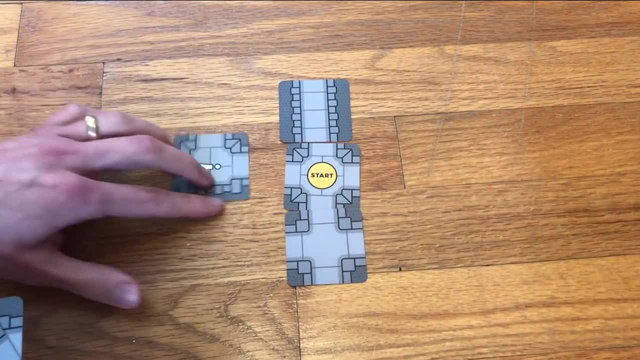 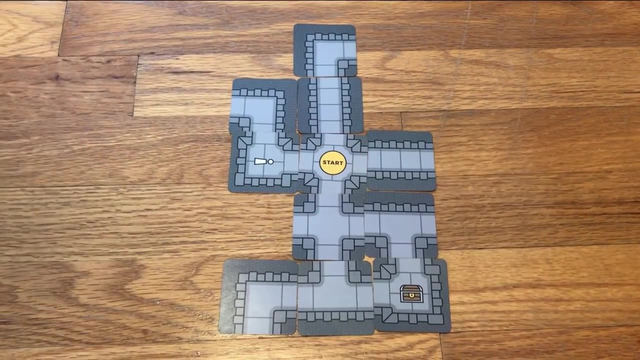 could implement to the game and how we can make it to be more focused as a party game and less as this grindy RPG. This ended up being the core gameplay that didn't really change much from this point, And that was that there was a 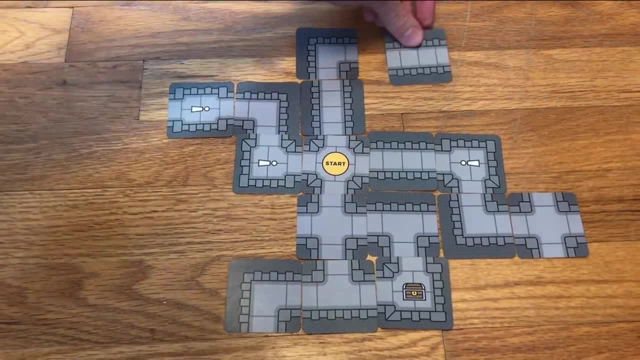 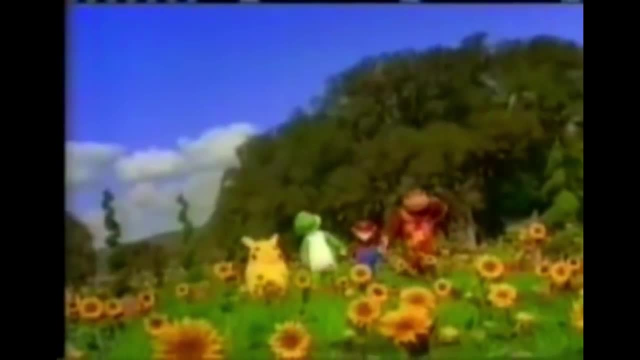 dungeon that the players had to build out And in this dungeon there were two cards, There was a key card and there was a gate, And the players had to find the key as quickly as possible. Now, before they find the key, all the 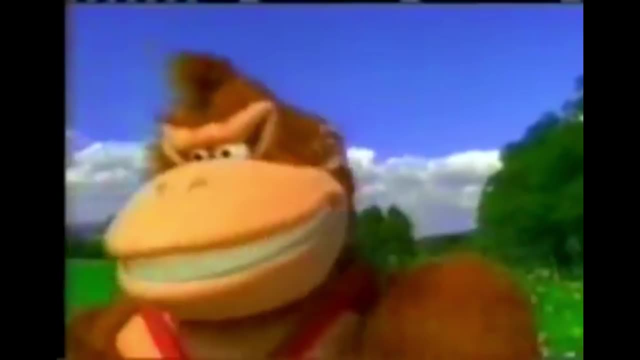 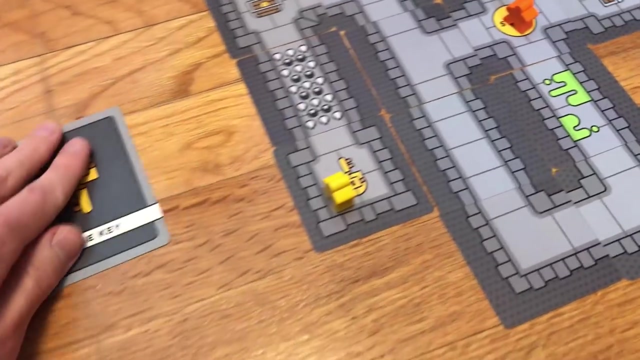 players are friendly and they can collect items by landing on treasure spaces, But after the key is found, all the players turn on each other And the goal is to be the first person to go to the gate tile with the key. And everyone plays as a unique character, and not just one, but two. These characters range in 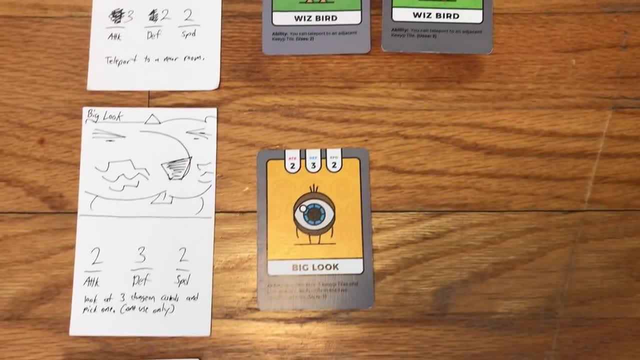 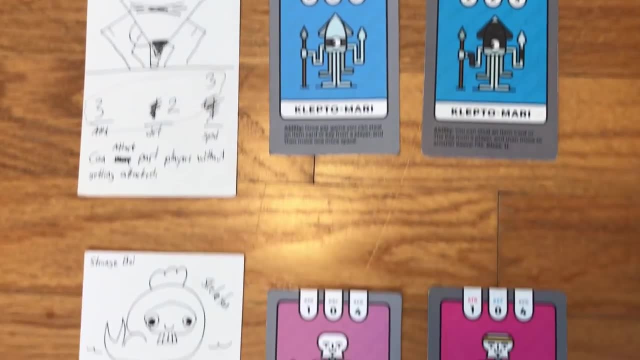 strength, defense, speed and even abilities, And that, paired with a random generation of the dungeon, made the game very different every time. It really felt like a multiplayer roguelike, but it was fun. Summer started to roll by and I was working on Fantasy World at the time. 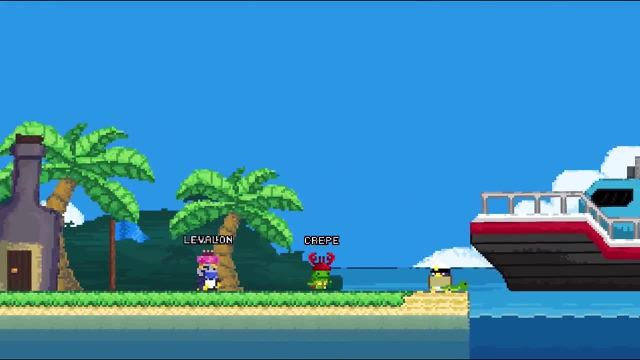 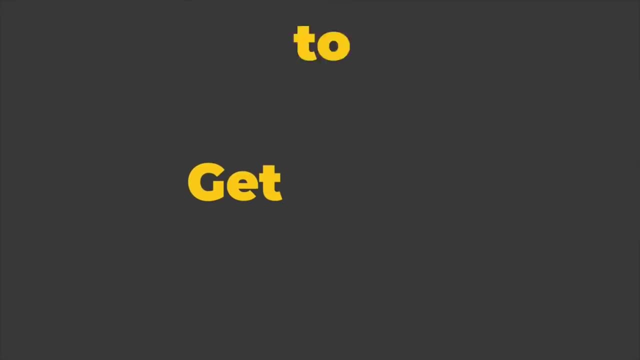 which is a side-scrolling 2D MMO. So, really, this idea of a board game sat on the shelf for a couple months, And it wasn't until the fall semester that year that I started to work on the game again, Before they were on the Firth team Bonzo. 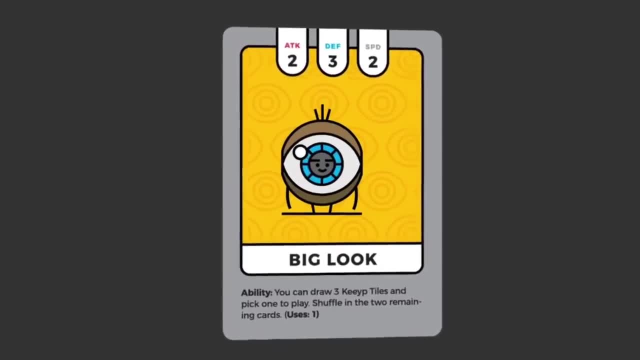 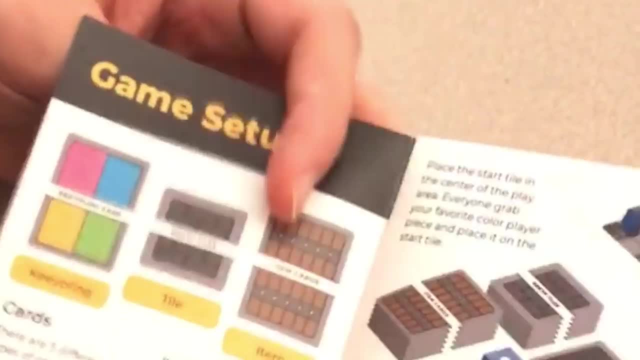 and Brad would actually watch me work on the game during class And before I knew it, Bonzo and Brad were a part of the team and were helping create artwork and assets and sketches. Eventually, after making some amazing character concepts in the game, Bonzo moved on to work on Fantasy World. I still was unsure what I wanted to. 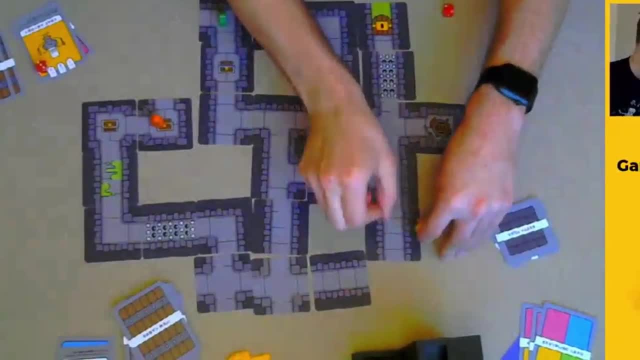 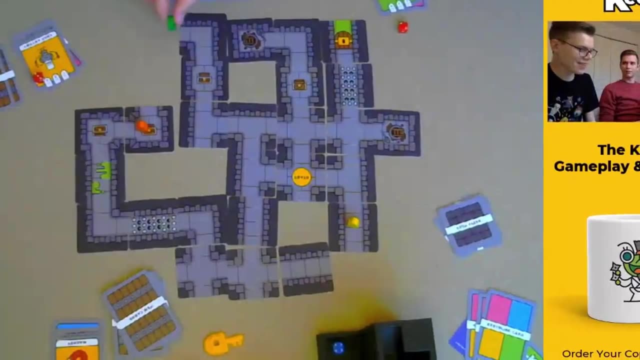 do with the game, and if it wasn't for the help of Brad, I don't think I would have been able to ever finish this game at all. At this point the game was pretty refined. We had messed around with different items, balancing characters, implementing more stuff. 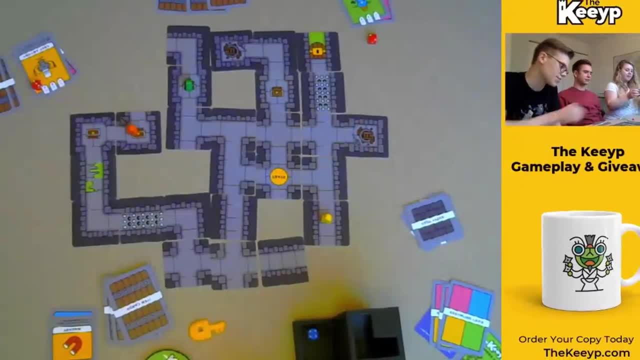 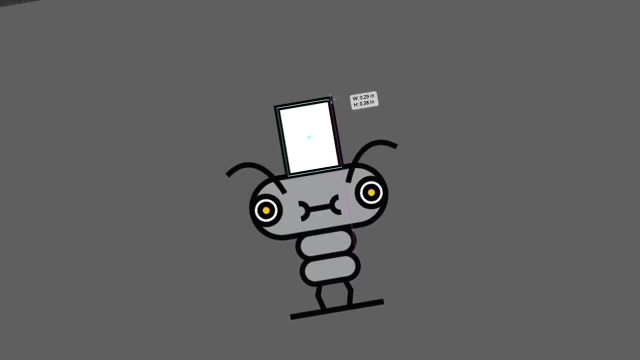 but the core mechanics didn't change at all. We also came up with a name for the game called The Keep, But majority of the work was just creating the artwork. I already established a style using thick vector outline artwork and Brad picked it up flawlessly. 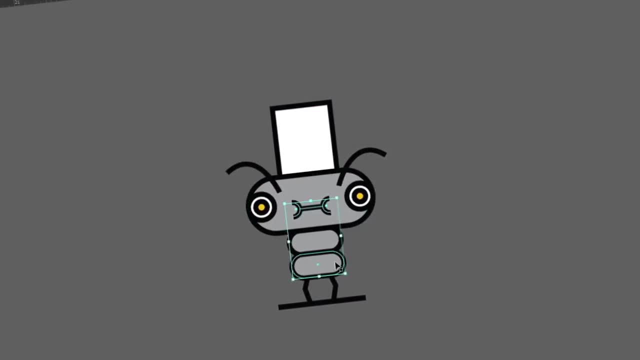 We also convinced some of our professors to let us work on it during school. If it was an animation class, we would make animations for promotion for The Keep. If it was a packaging class, then we just used it to design the packaging for the game. But the game wasn't. 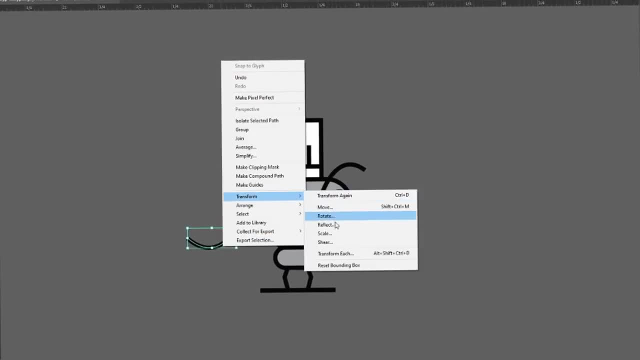 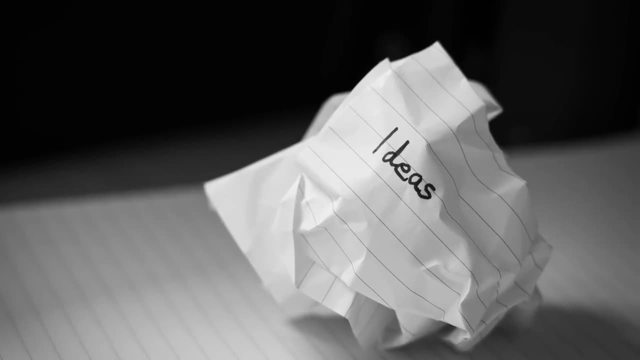 finished yet, so we decided it was time for us to set a deadline. The game needed to go out January 1st 2018.. Being only a couple months away, we started to brainstorm our marketing plan. Most people, when they want to publish their games, put it on something like: 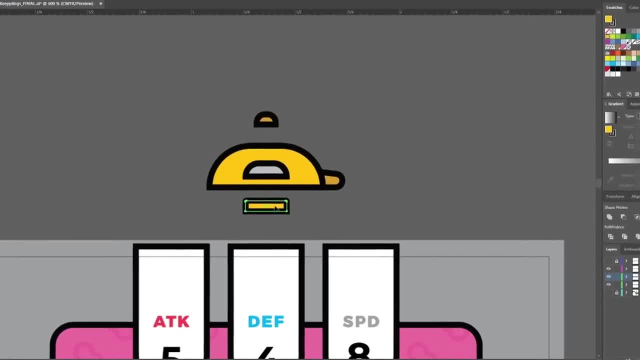 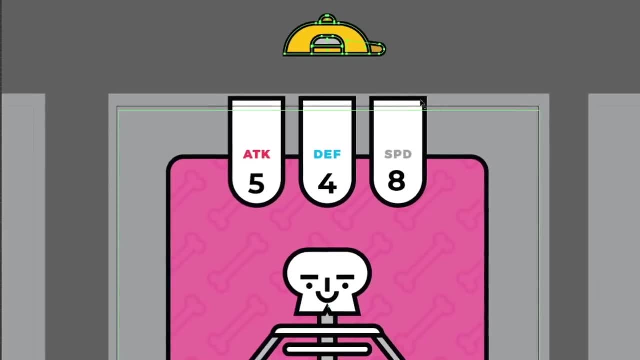 a Kickstarter. But for us we didn't know if we had enough people to successfully launch a Kickstarter, So we figured we would do our own pre-orders. We figured we would make a shop, people could place their orders and at the end of January we would buy as many copies as we could. 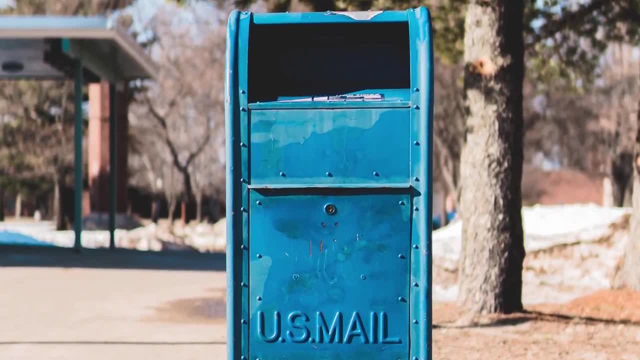 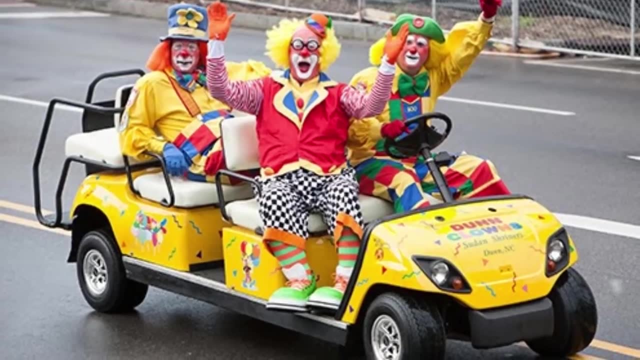 and then ship them out. But instead of actually mailing out copies, we actually drove to as many places as possible to hand deliver them, just so we could save on shipping costs. But we knew before we launched it we needed to generate hype, So we decided to have a little. 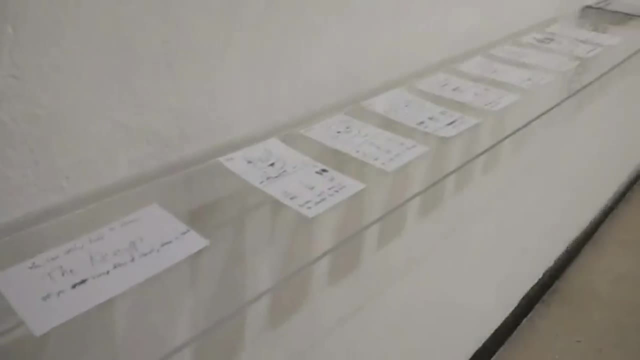 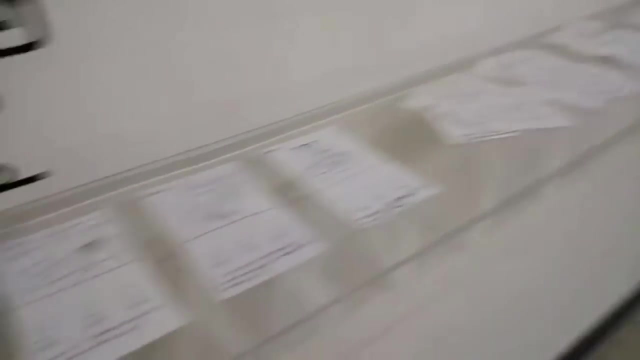 gallery show at our art school show off the process of how we made the game, show off some merchandise that you could buy there, and we even had a game night so people could come and actually test the game before it came out. We were also doing weekly live streams on Facebook to generate 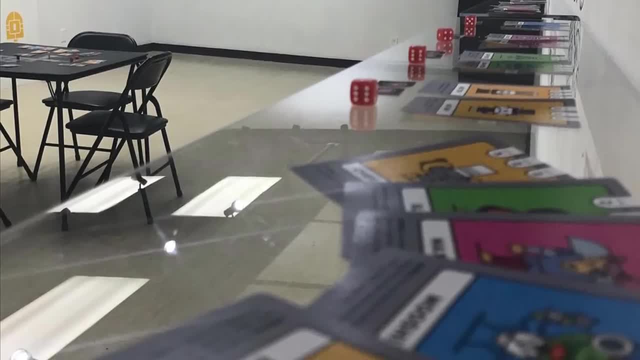 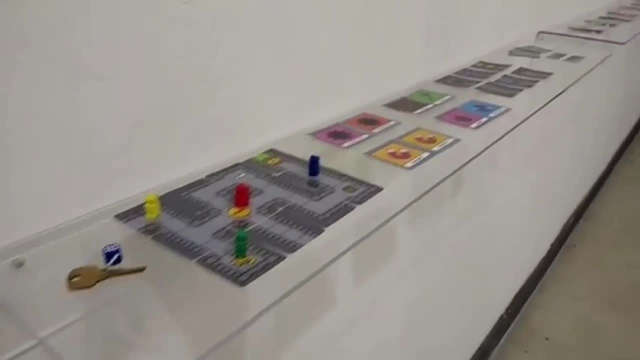 hype and it was amazing to see how excited people got about this little board game. So when January 1st came by, we were surprised to see how quickly we got funded. With our first round we were able to sell enough copies to buy actually extra and pay for the next batch. I'm not 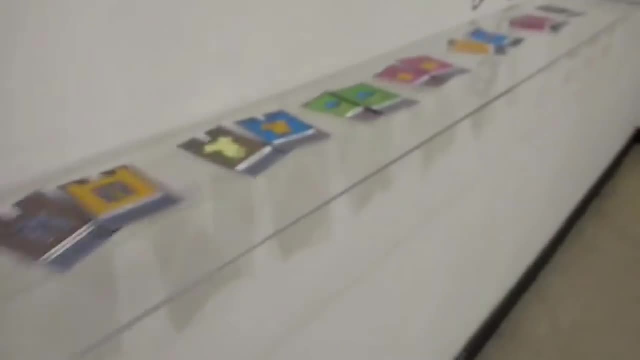 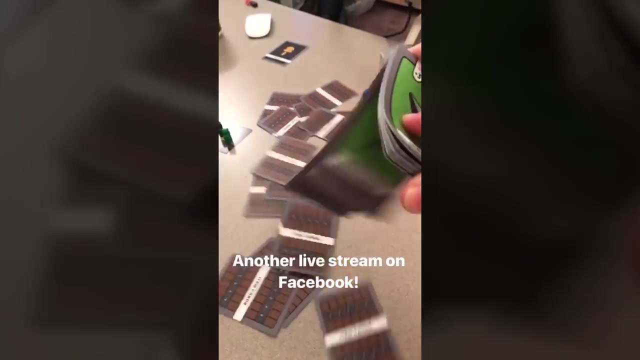 going to lie, that was one of the craziest years of school, considering it was our senior year and we should have been more focused on- I don't know- actually working on schoolwork and not releasing a board game. But it was an absolute blast to see the smiles of satisfaction people had when 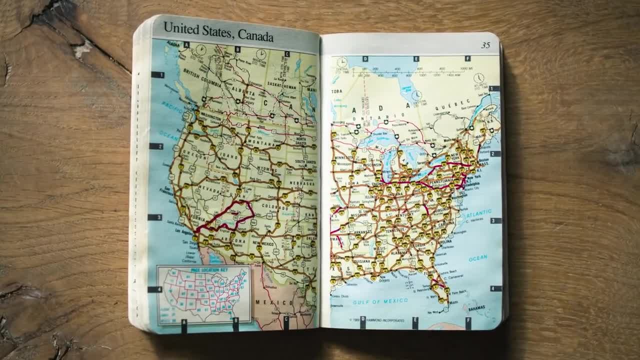 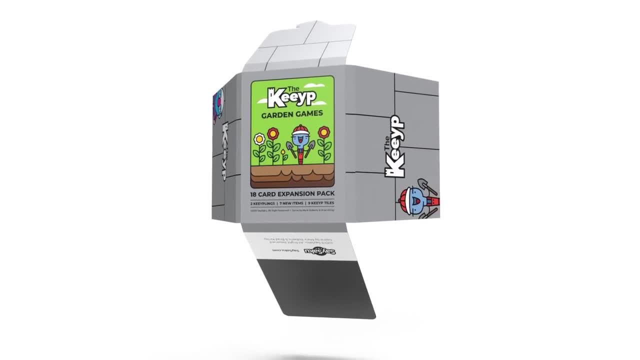 playing the game. Now, to fast forward to the present day, The Keep has been sold in over 15 states. Some people have even brought it into Canada. We also created expansion packs that really added to the gameplay And, to be honest, I still feel like there's so many expansions we. 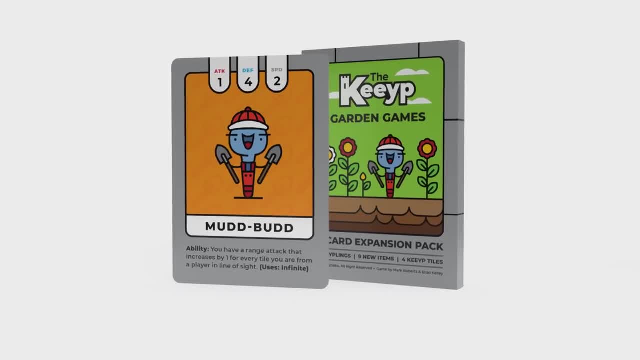 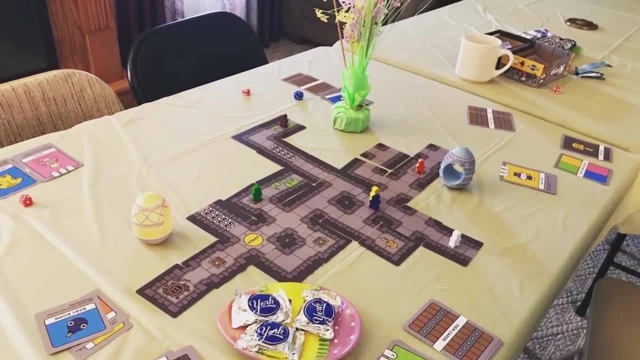 can make to really add life to The Keep. It was also so cool to see the impact that The Keep had on other people's lives. There was a family that would play The Keep every single morning with their kids before they started their day. There was another person that used The Keep to teach strategy and rules to special needs. 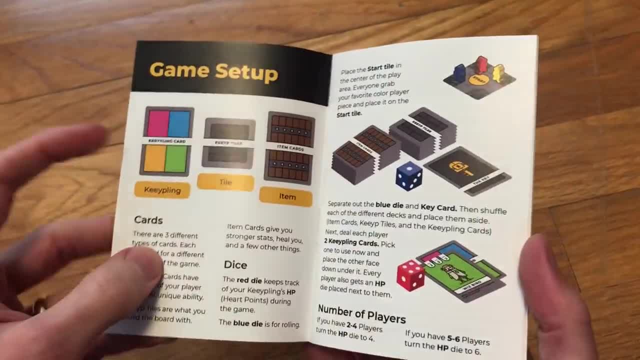 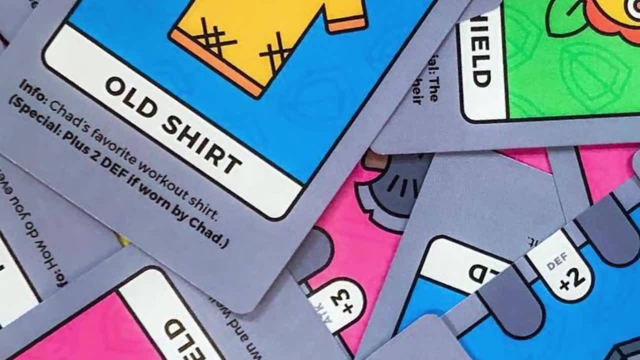 kids, And also one of my friends I grew up with, who is a huge cynic and hates everything, said it was the best board game he's ever played And even though it has some flaws and it's not a perfect game, it still, to this day, is my favorite board game, And I know that may sound strange. 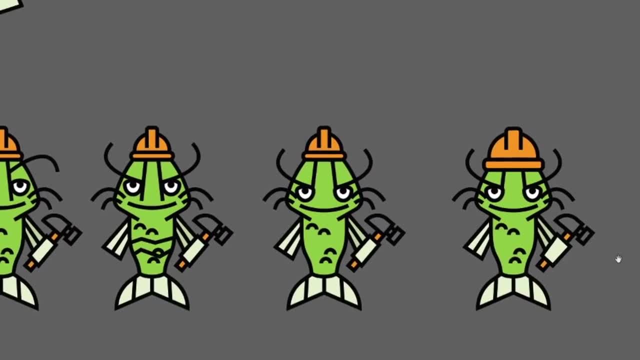 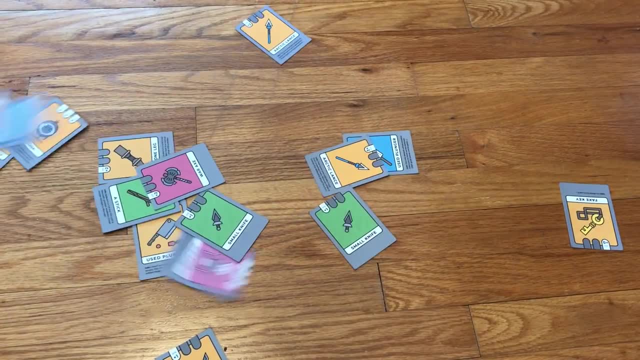 but I did it. I achieved the dream of making a game that I loved and I want to play. But not only that, but I made friends along the way. I was able to reach out and talk to new people in our community, And it was just so cool to see the love and support of the people around you that wanted 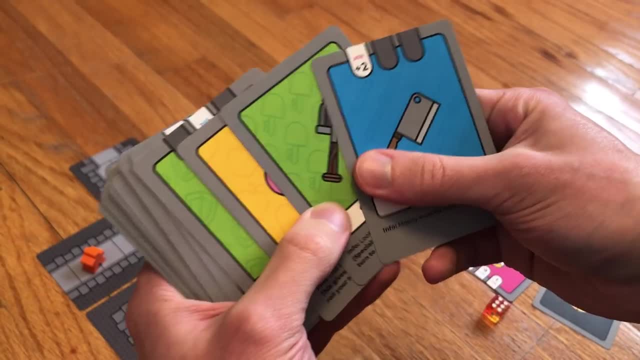 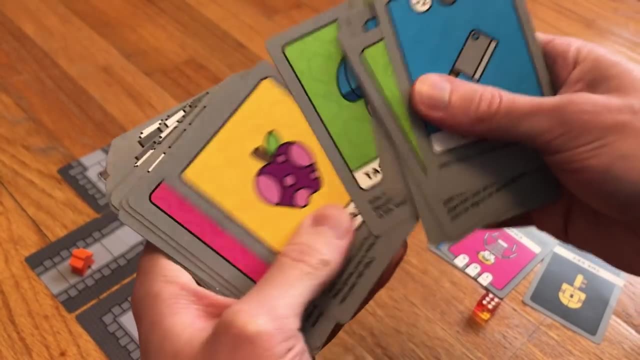 to see you thrive and be successful. Now, the only sad part about this story is that board games are expensive to produce and that we really didn't make any profit during The Keep's lifetime. It was a lot of work for not a whole lot of reward. 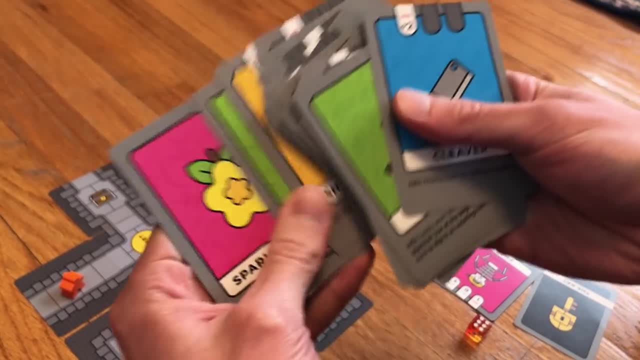 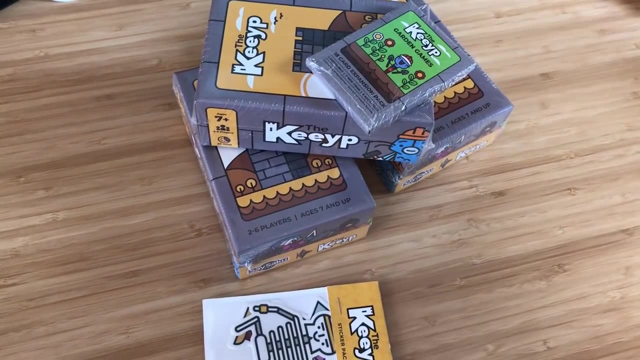 And that also means that when we sell out of our last copies- which we only have about 20 or 30 left- that we probably won't be reprinting it anytime soon, unless we're contacted by some publisher or there's enough interest. So if you're interested in getting a copy of The Keep for yourself.